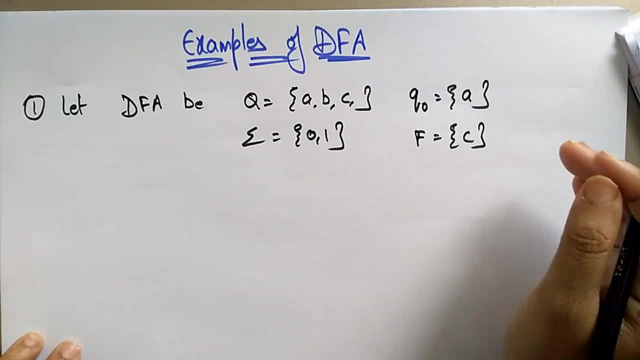 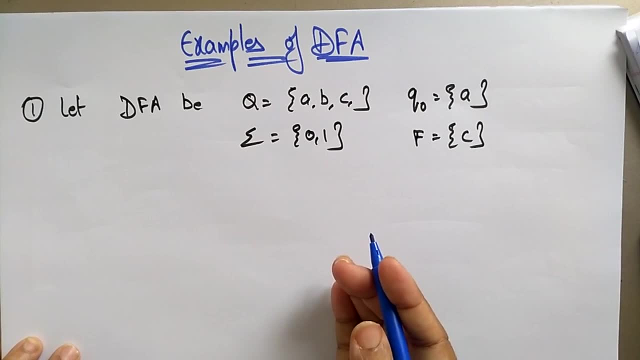 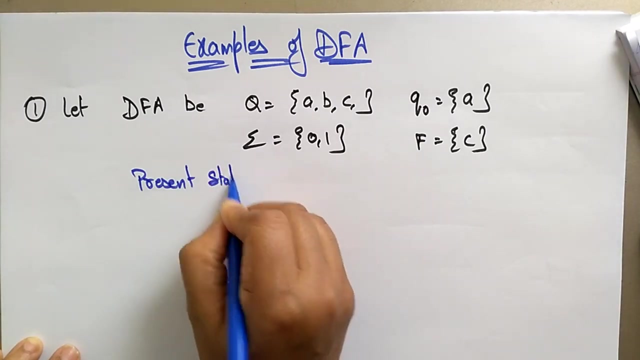 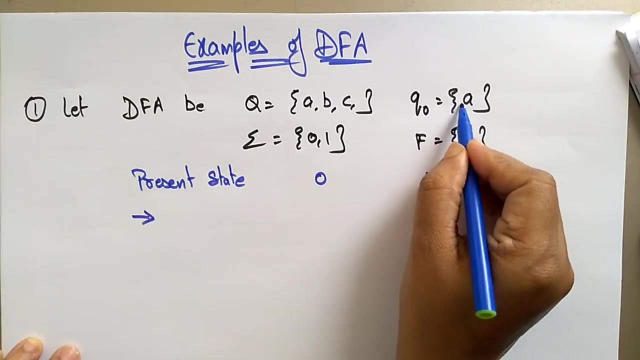 and what they are asking. they are asking: the transition function of the table is also they given. we need to construct the state transition diagram for that. so the present state: they are given the table. so input a 0 and 1, so initial state starts. what is the initial state? 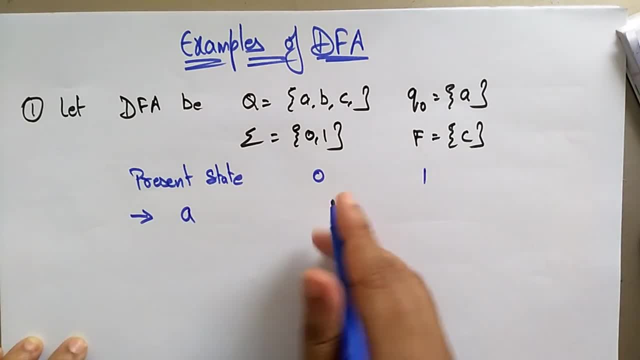 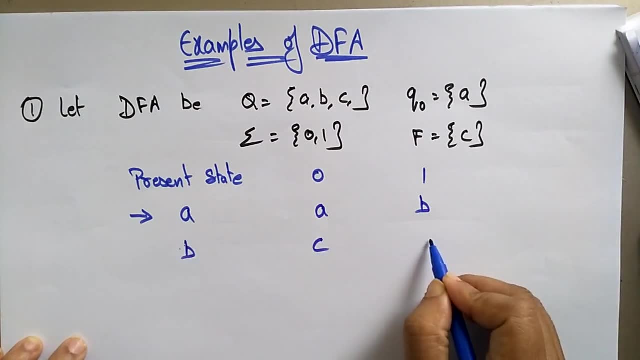 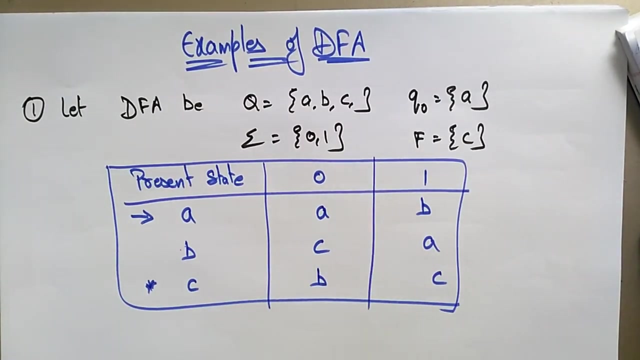 a is a initial state, right. so a on 0 they are given as a, b and next state is b, c, a and the final state is represented with star or double circle: b, c. so they are given a transition table. now by seeing this table you can easily construct the dfa for this table. so you have to remember. 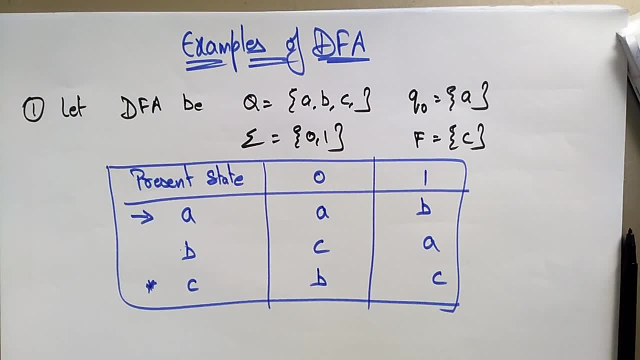 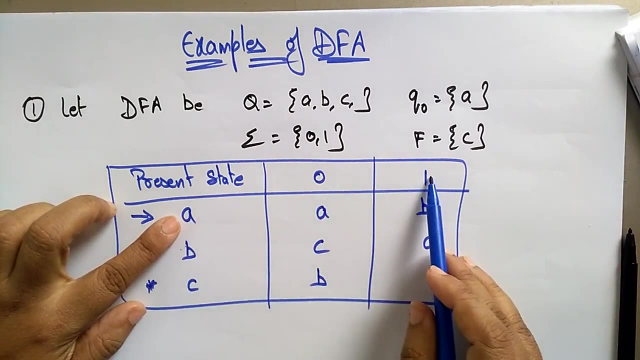 that in dfa only one path which is going to that particular input. if you are taking any particular input, only one path will be going to that particular input. okay, so the a can be on zero, it goes to only a, or it can on one, it goes. 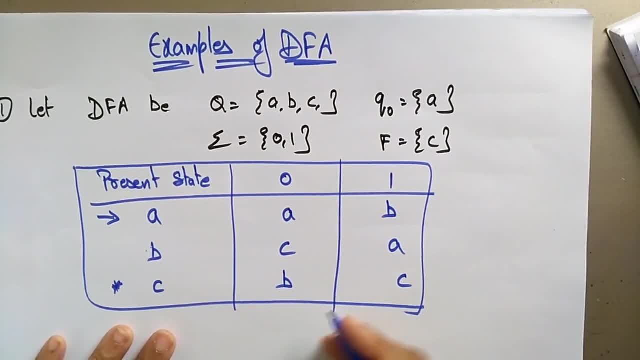 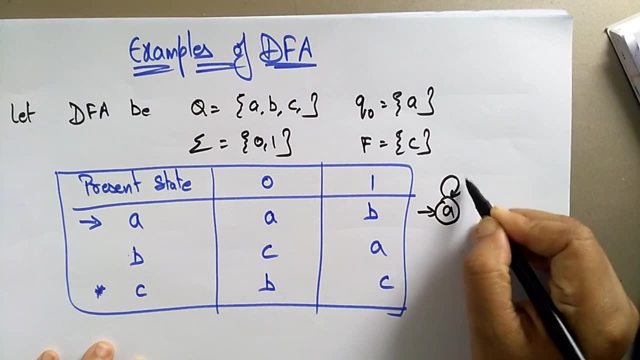 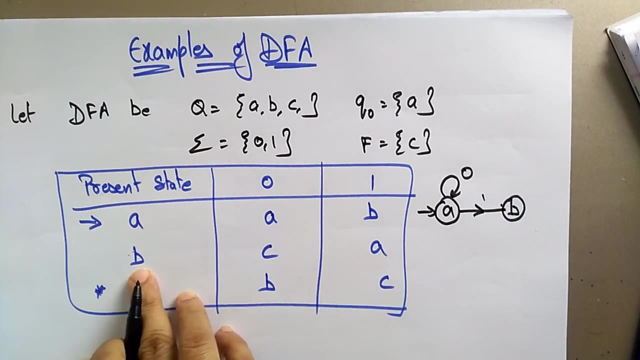 to only on, only on to b. so here let me draw the diagram. what is the initial state? is a, so a on zero? it goes to a, only a on one. it goes to b. now coming to b, b on zero goes to c, so b on zero. 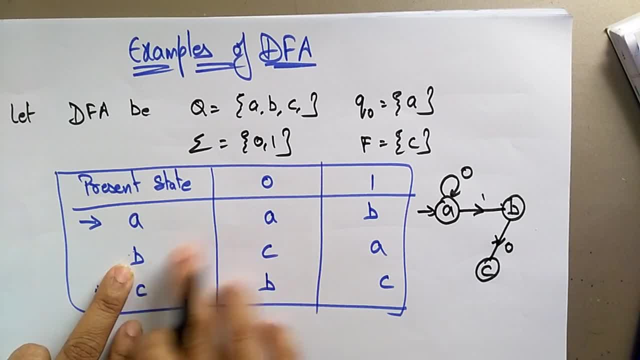 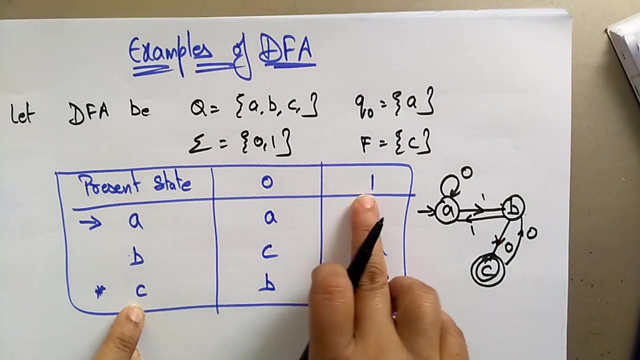 goes to c, b on one goes to a, b on one goes to a. okay, b on one goes to a. now, coming to c, c is the final state and c on zero goes to b. so c on zero goes to b and c on one goes to c itself. 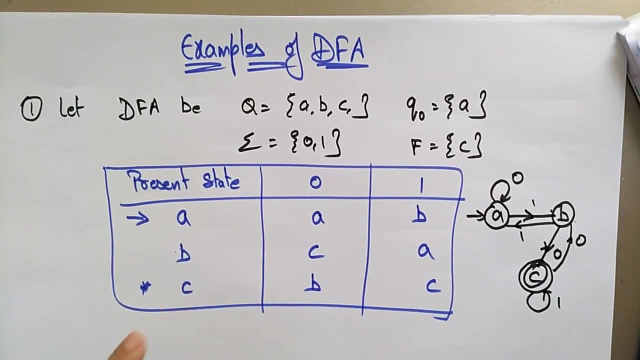 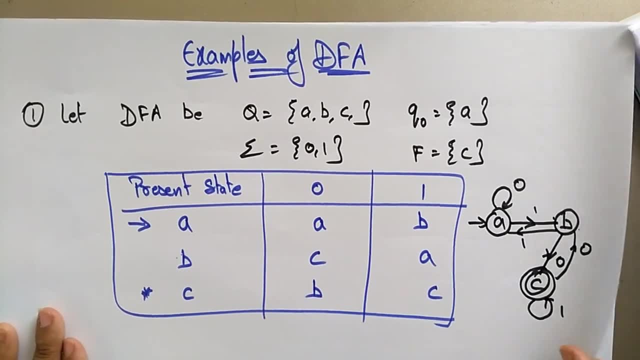 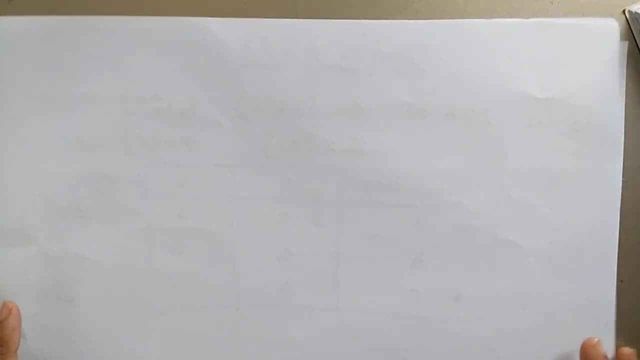 so this is a state transition diagram for this for the given table. okay, this is one way of asking the question, so let me take another way. so i'll try to cover almost all the types. means the different ways they are asking the question, because every one of them is asking the question. so i'll try to cover almost all the types. 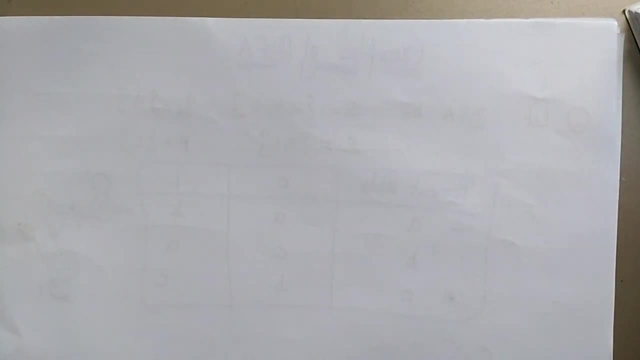 every student is getting confused. what is this question? how can what i have to draw and what i have to be implemented so at the same pattern means you can easily recognize. but let's see the different patterns. let me take the another example too. it's the another way of asking the 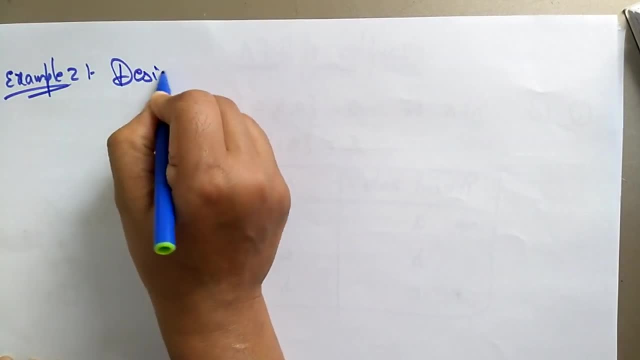 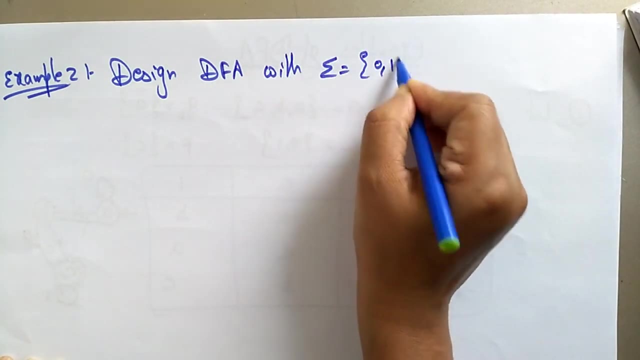 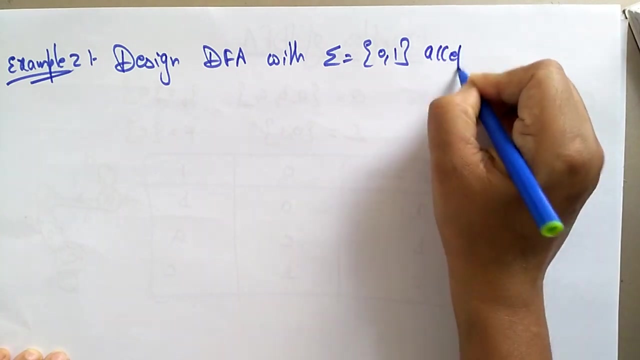 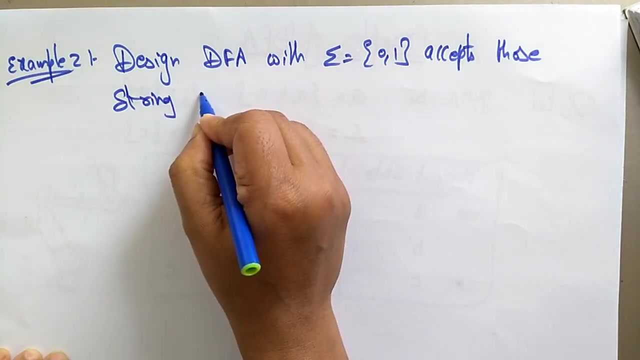 question. so here they are giving the question, like design dfa, i need to design dfa with. they are given sigma zero, comma one. a sigma means set of alphabet, means input symbol, serve zero one and it has to accept this input symbol accepts those string, those string which starts. 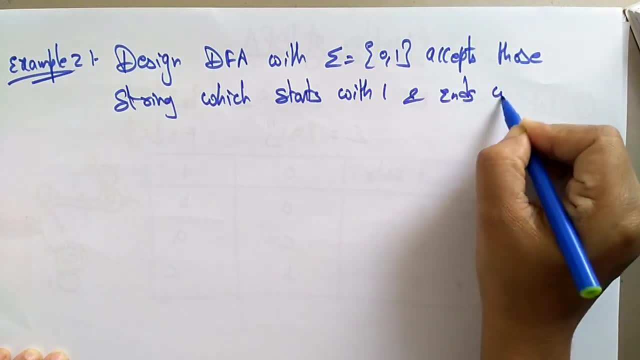 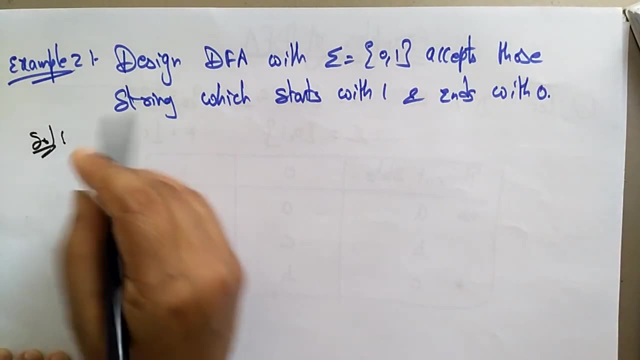 with one and ends with zero. so they are asking that, uh, the string, set of string will be there. that string would: uh, starts with one and ends with two. so they are asking: each string is going to the left, vitality Нет were going to the right. one going to p is not going to be having none floating by any means. that's why it is still the same. 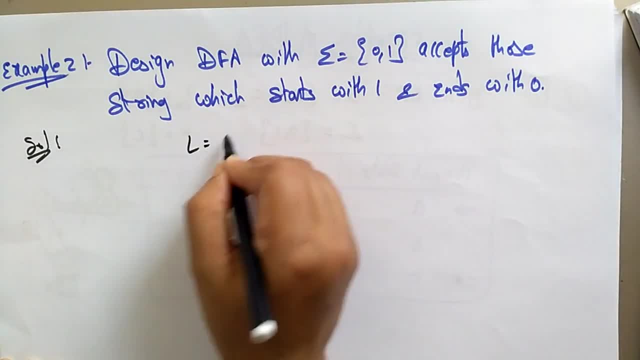 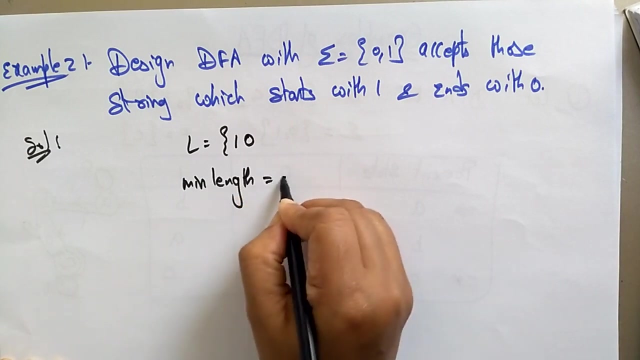 0. So compulsorily it has the language, whatever we have taken that string has to. starts with 1 and ends with 0.. Starts with 1 and ends with 0. So the minimum length of the string here is 2.. Okay, So the minimum length of the string is 2.. It's a minimum length, or? 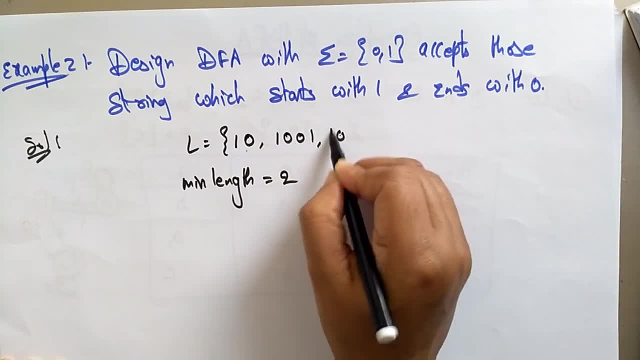 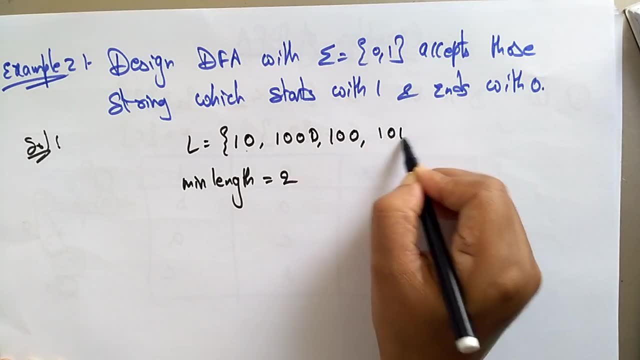 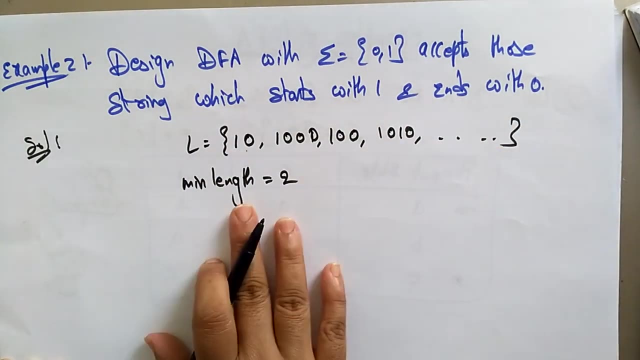 else you can. starts with 1 or ends with 0.. Starts with 1 and ends with 0.. Starts with 1 or ends with 0. Means like this, So it should be anything the length of the string. they are not given the maximum length, but the minimum length is 2, compulsory because 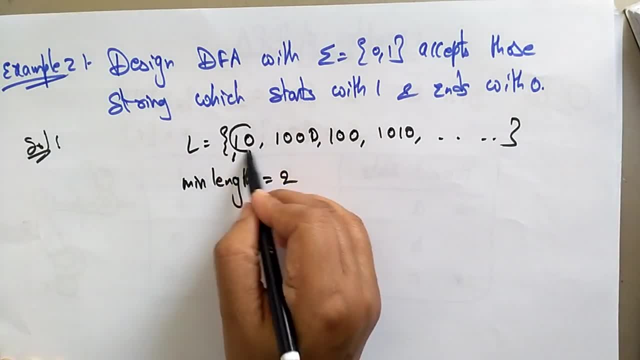 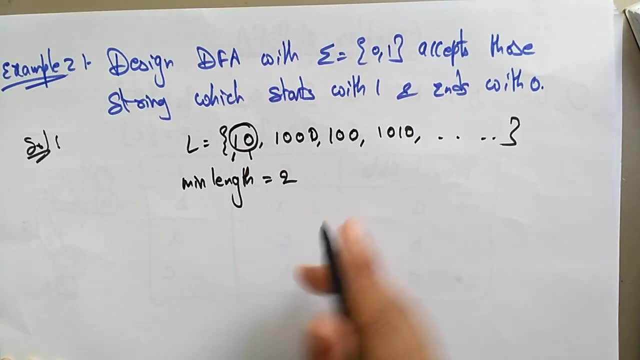 the string should starts with 1 and ends with 0. Means the two characters are there, Two symbols are there, So the minimum length of the string is 2.. So, whenever the minimum length of the string is 2, is the number of states or the number of states that are participate? 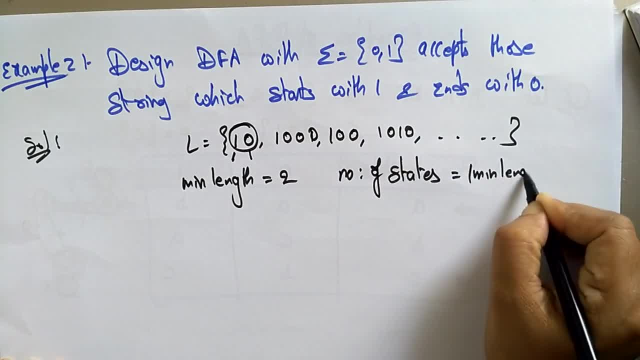 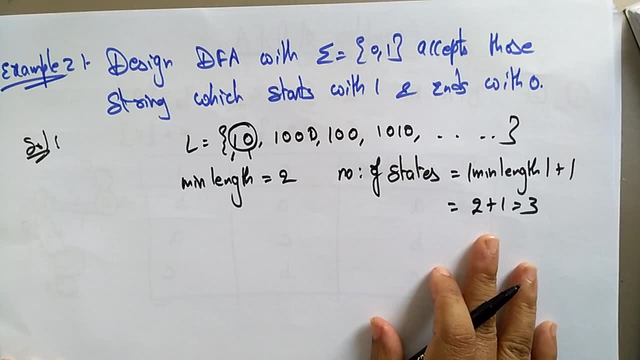 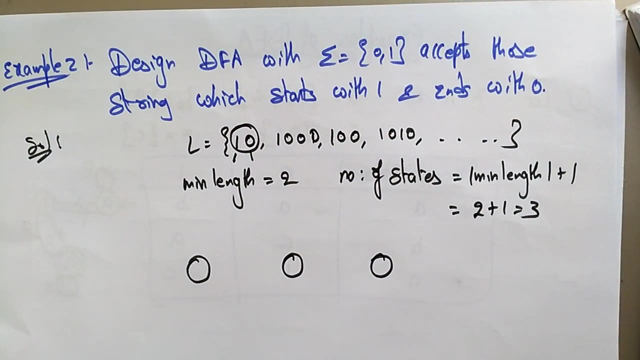 in the diagram is minimum length plus 1.. So what is the minimum length? 2 plus 1, that is 3.. So number of states are 3.. So let's take three states. Okay, So now I want to construct the DFA, or the deterministic finite. 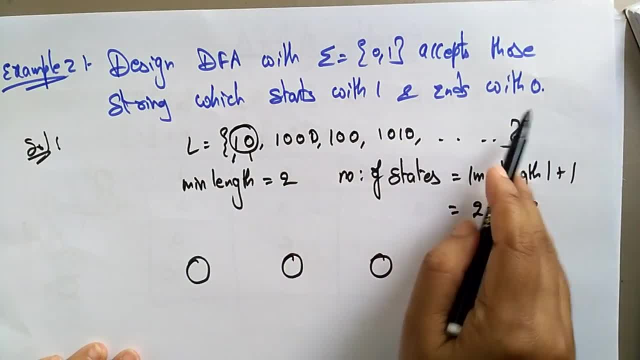 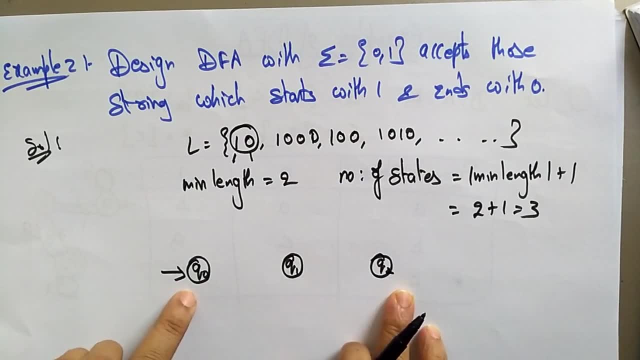 automator with this inputs and that string starts with 1 and ends with 0. So here this is the initial state. Let's take Q0, Q1 and Q2.. So three states I have taken. Let's take first minimum. 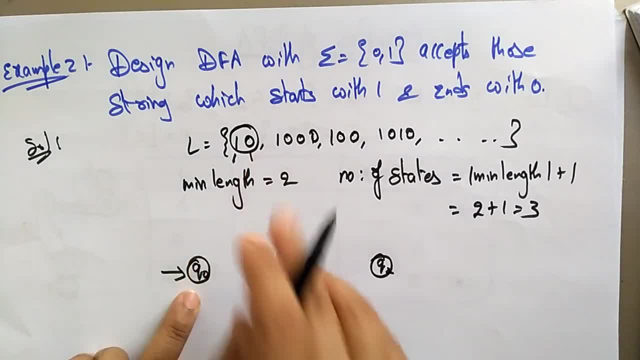 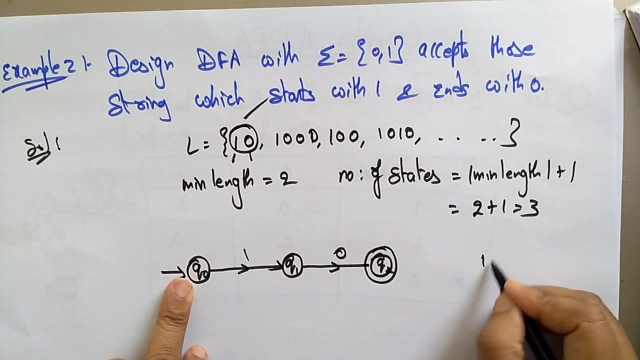 Minimum string. the starting string starts with 1 and ends with 0.. Starts with 1.. So Q on 1 goes to Q1 and next it has to. this Qt is the final state. on 0 goes to Q2.. So the first string is accepted. Q on 1 leads to Q1 and Q1 on 0 goes to Q2.. So 1, 0. So. 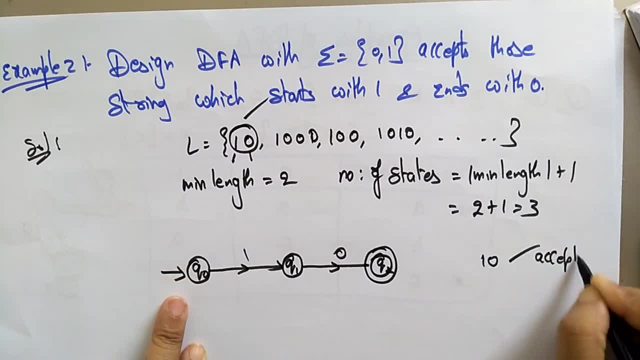 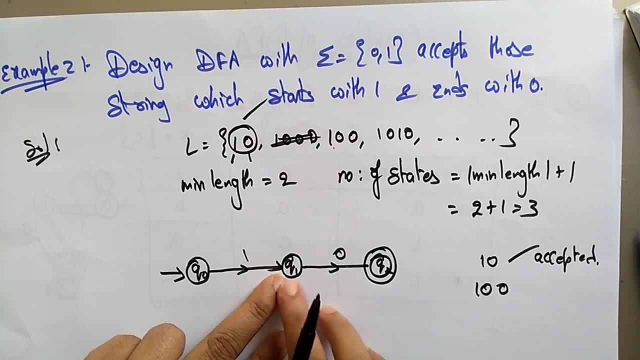 the 1, 0 it reaches the final state means it accepted. Let's take, suppose Let me take this second- 1, 0, 0.. Is it accepted or not? I have to take, I have to check. So Q on 1 goes to Q1. So let me take 100. So Q1. next Q on 0, 0 and again. 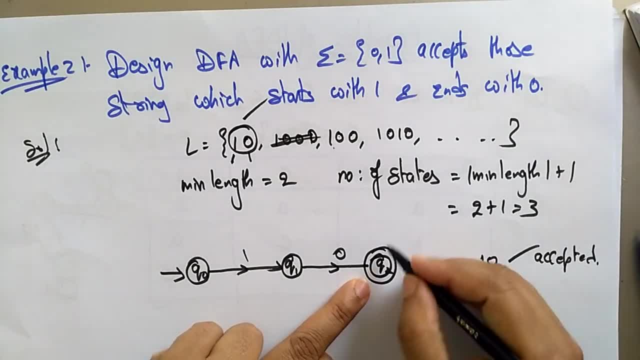 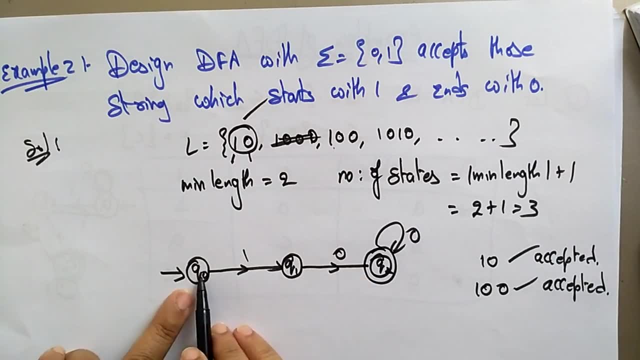 the 0 has to become. Let's take this loop. So now this is also accepted. So Q on 1, 1, 0, 0.. It reaching is we have to reach the final state, okay. so next let me take this string: 1 0, 1, 0, the our question. 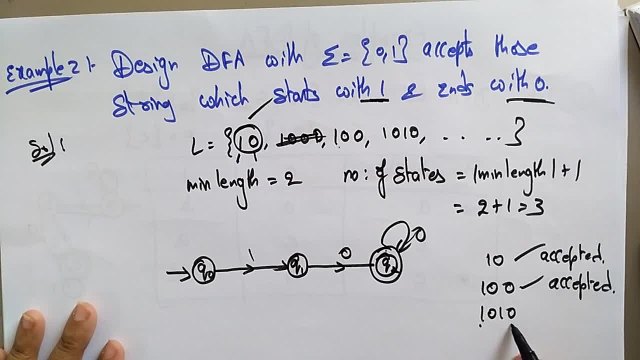 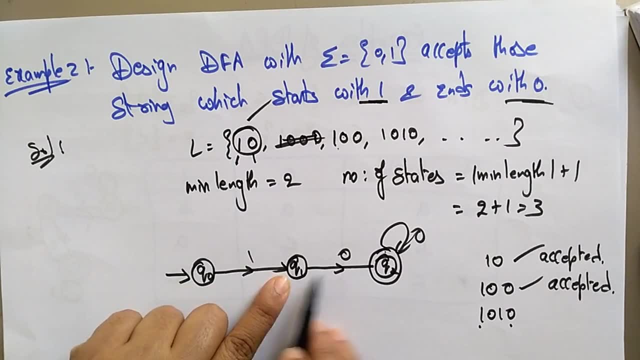 is, starts with 1, ends with 0. so here i starts with 1 and i ends with 0. so in between, whatever it may be, let's check: q: naught on 1 goes to q1, q1 on 0 goes to q2. so again, q2 on 0 goes to. 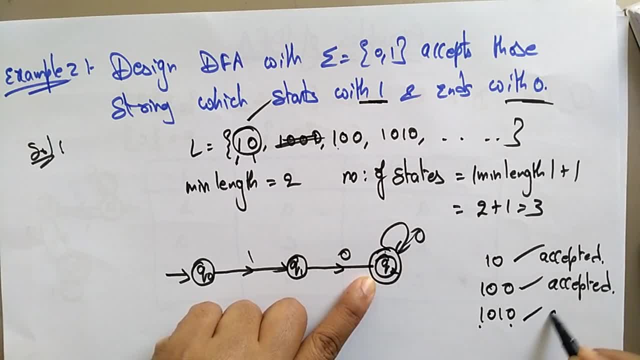 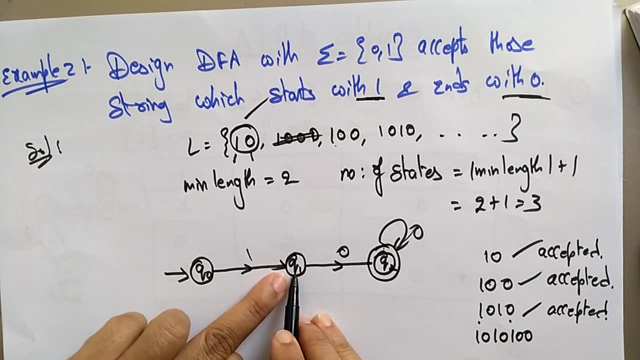 q2 itself means it is reaching the final state accepted. so this time let me take 1 0 1 0. 1 0 0. let me check this- is it accepted or not? means in this way you need to be checked. so q naught on 1 goes to q1 0, q2, q2 on 1. so again it has to come like this: q2 on 1 goes to q1. 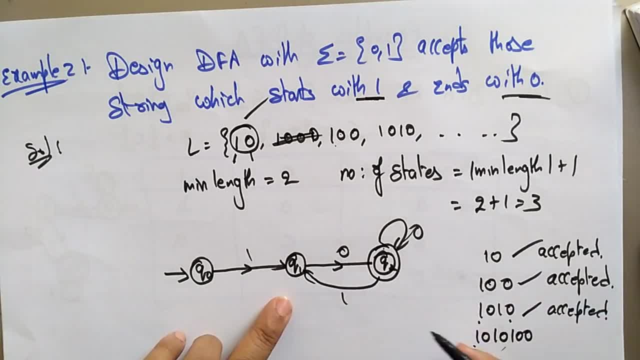 and q1 on 0 goes to 0, like this. so like this we have to be checked. so the here how i am going to construct the dfa. the dfa means each state has to go either 1 and the 0, so here it is going to 1 and here the q1 is going to 0.